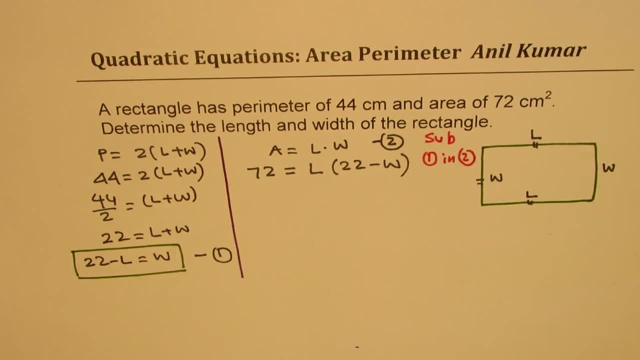 So we get one equation: Sorry, So L, right, So okay, So that's our equation. Now you can actually solve this equation and get the result right. So we get 72 equals to 22. 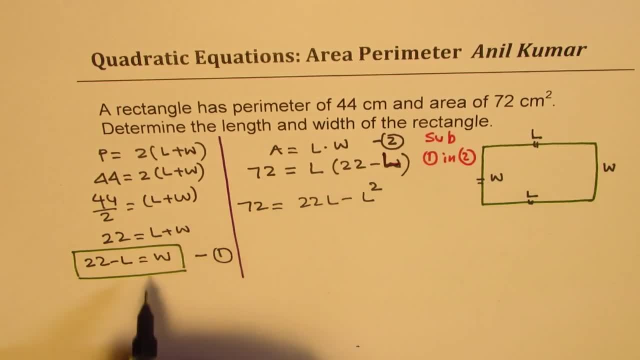 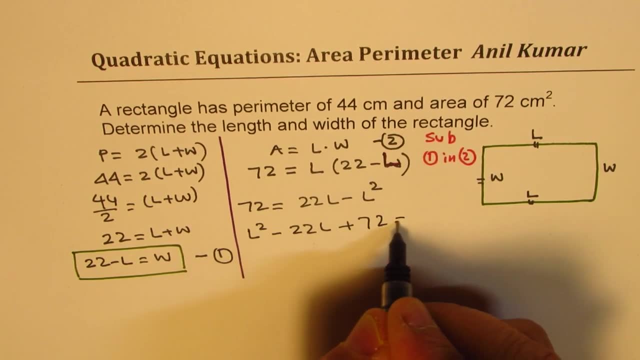 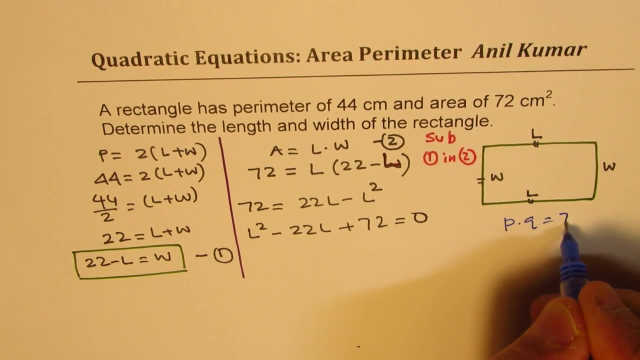 L minus L square right, This is length- Length. Bring them together: Length square minus 22. L plus 72 equals to 0.. Now factor: We are looking for product and sum. So let's two numbers whose product is 72 and their sum should be minus 22.. So what are these? 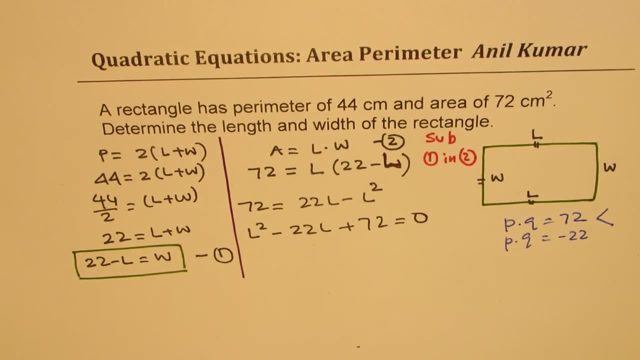 two numbers. This is what you need to work out, right? So if it becomes difficult, what you could do is you could just factor 72,, right? So if you factor 72, we could say, well, 72 is what. 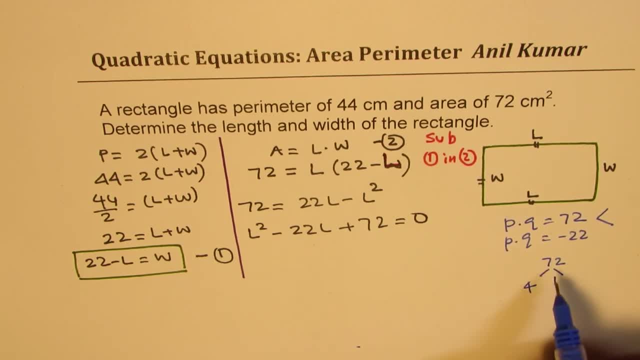 If I divide by 4, I get 4 times 1 and 4 times 8. And you see, when you add these two, you do get 22,. correct Now, since we need negative, so both should be negative. It doesn't make. 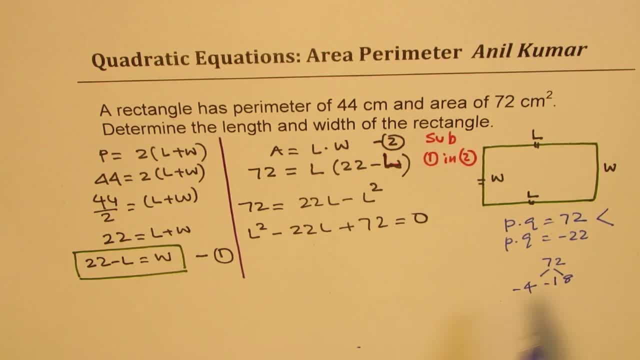 sense to you correct. So that is how you could factor. So we have two numbers. So we can now write this as L minus 4 times L minus 18.. It should be equal to 0. So that. 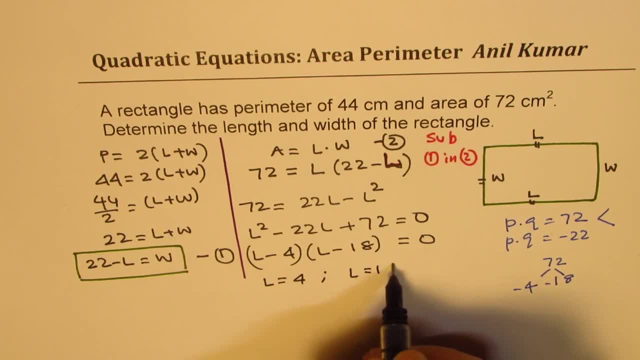 gives you two solutions: L equals to 4 or L equals to 18, right. So these are your two solutions. Well, if I substitute 4 here, then I get W as 18, right? So if I write: 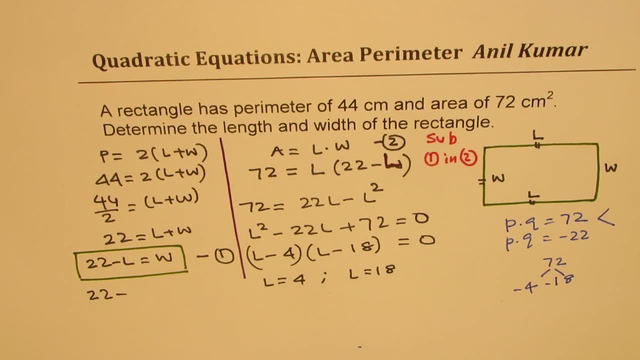 let's say, if I substitute 18, length, we want bigger one, right. So let us say which one. We take this one right. So if I do 18, I get this as 4 equals to W3, correct, So that. 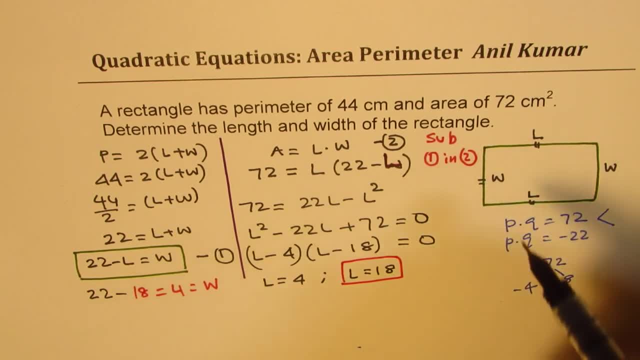 could be one combination, It doesn't matter what you call one as, But anyway, we know one of the sides is 18 for us and the other side is 4 for us, correct? So that gives you the solution And our answer is that the length- normally we put longer side for length.